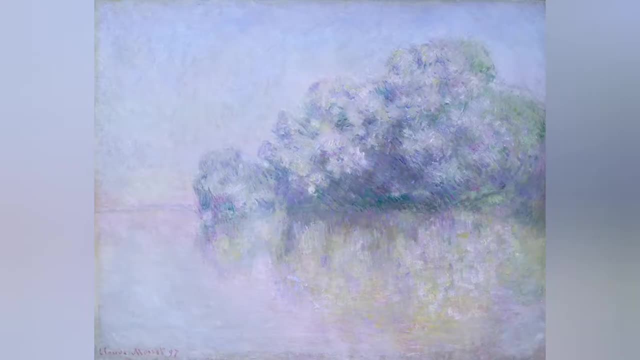 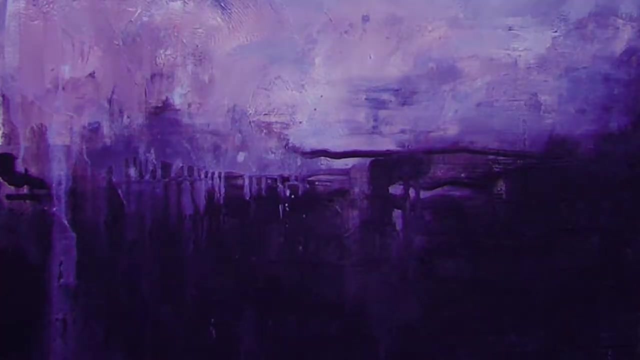 shade of color, but as something more luminous, Perhaps a purple lit from within. Violet is the shimmering, fugitive color of the sky at sunset. purple, the assertive, substantial color of imperial robes. The plants can be poisonous when ingested due to naturally occurring toxic. 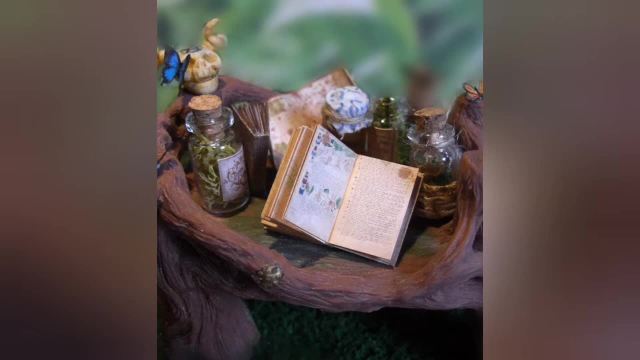 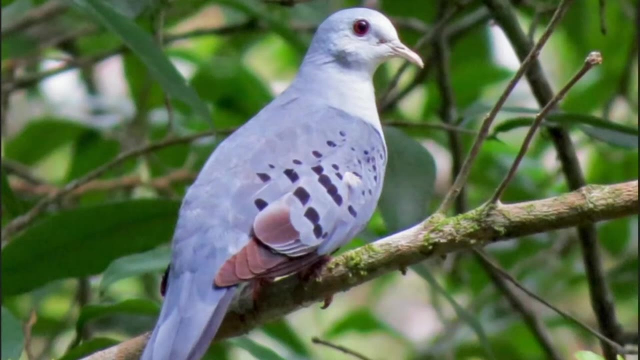 alkaloids. The flowers were used for their astringent and tonic properties in early medicine. There are other names for periwinkle, For example. the French phrase poul de roche means rock dove. The moniker was for the blue resembling the color of a dove's feathers. The plant goes by other 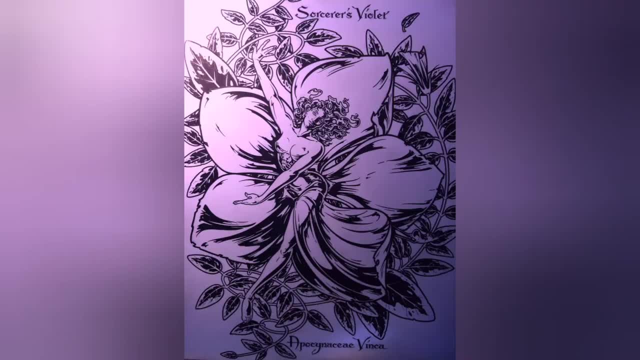 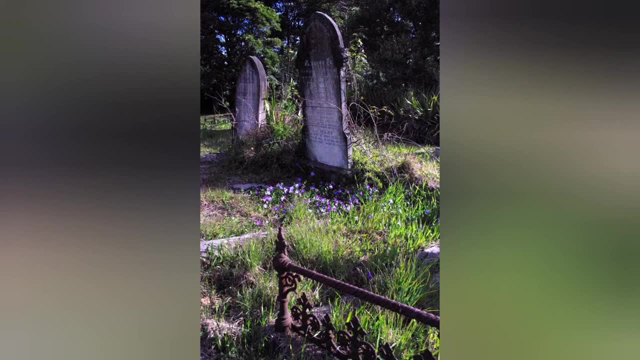 names as well, like the devil's eye, joy on the ground, sorcerer's violet flower of immortality and death's flower. The plant is known as death flower because it often grew in cemeteries. They were grown as bedding flowers, as an ornamental plant for a damaged or missing marker. 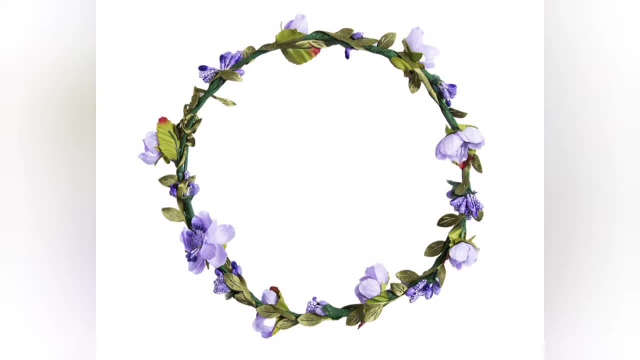 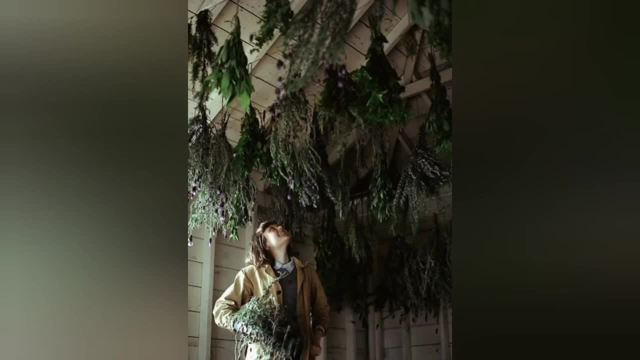 In Italy and England, the flowers were woven into hair bands for children's funerals. In medieval England, the flowers were made into garland for condemned men sent to the gallows for execution In witchcraft practices. periwinkle flowers are said to banish negative energy and 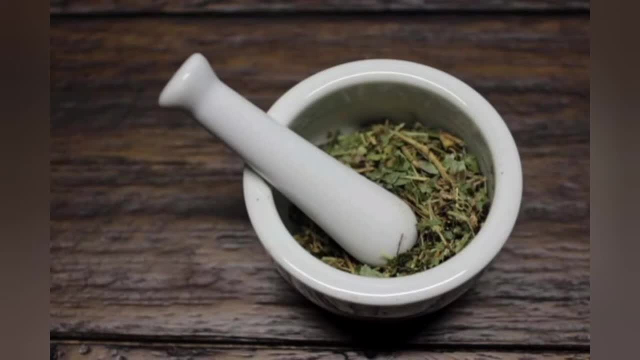 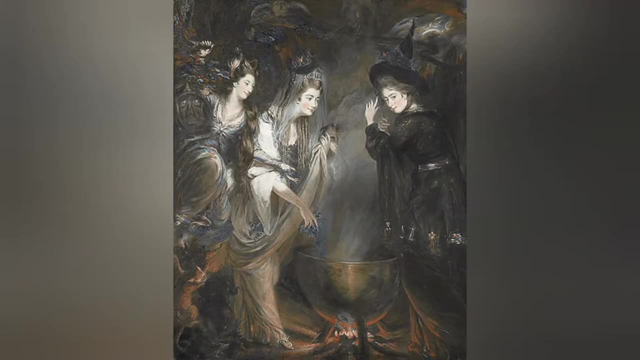 restore mental clarity. Periwinkle allegedly protects people against evil spirits, the devil demons and necromantic magic. Periwinkle was also used to make charms and love potions In Welsh folklore. if you pluck the periwinkle flower from a grave, it will bring you bad luck. 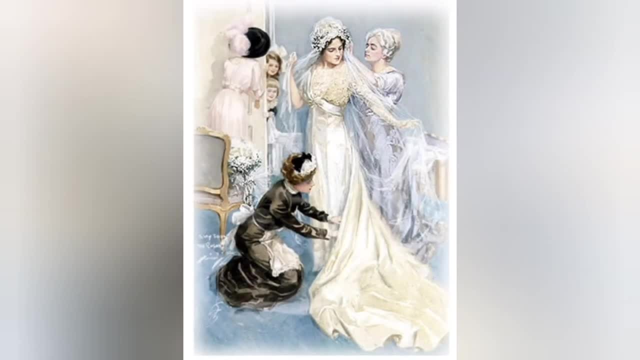 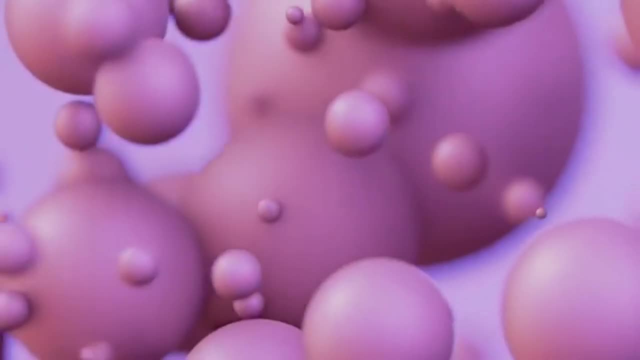 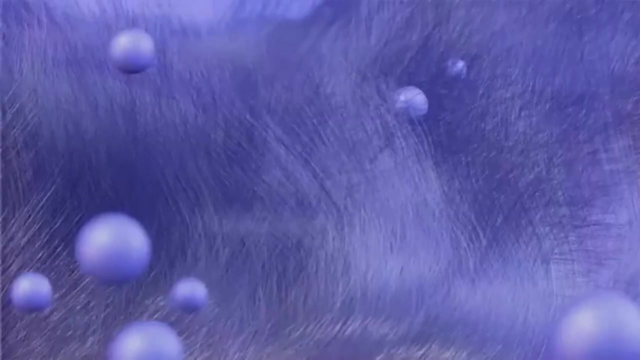 and have you haunted by the grave's owner. The flower is also sometimes associated with marriage and may have been the something blue in the traditional wedding rhyme. Pantone, known for their universal color match system, has just announced the 2022 color of the year as Very Peri. According to their press release, it is a new Pantone color whose 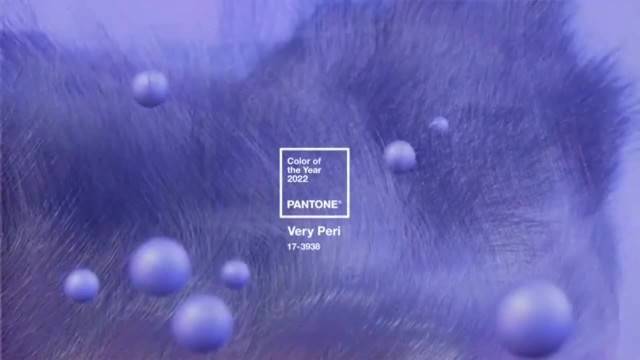 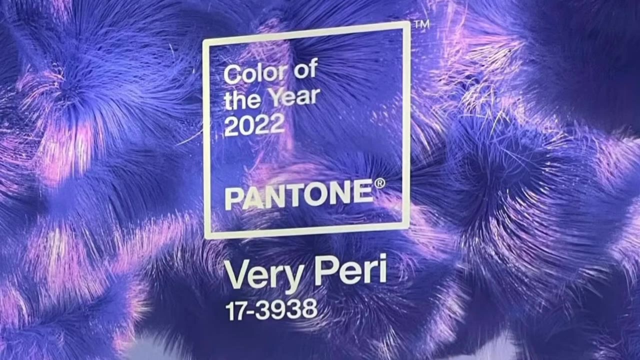 religious presence encourages personal inventiveness and creativity. Very Peri is a symbol of the global zeitgeist of the moment and the transition we are going through As we emerge from an intense period of isolation. our notions and standards are changing and our physical and digital lives have merged in new ways. 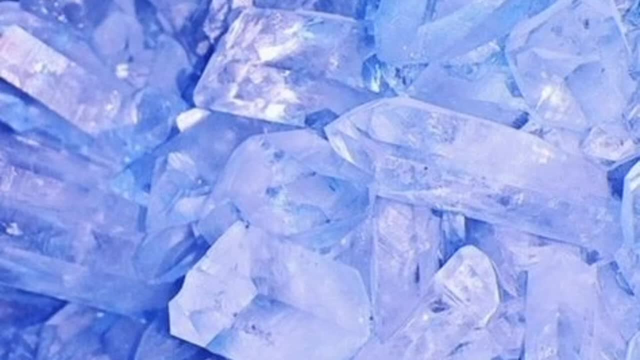 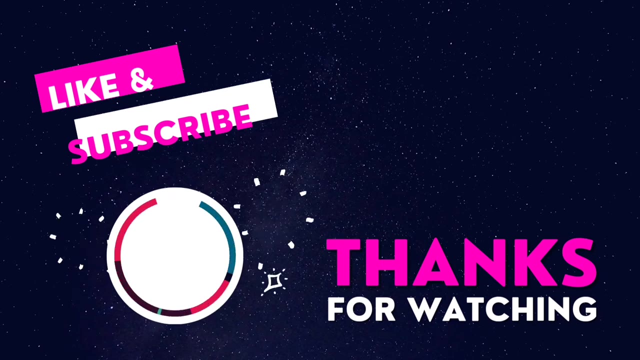 Today, Periwinkle's muted hue invokes feelings of serenity, optimism and lightheartedness. I hope you enjoyed this video. If you did, make sure to like, comment and subscribe to the channel. I'll see you in the next one.